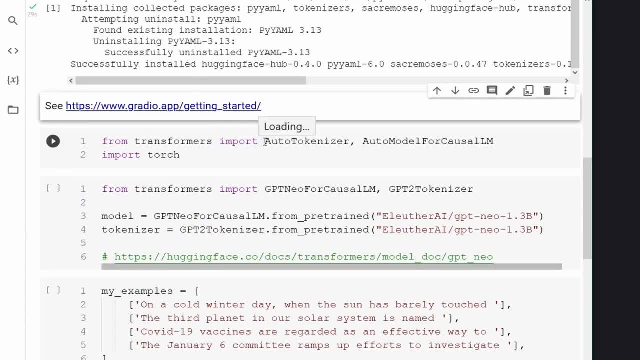 And then from the transformers we have our auto tokenizers and our GPD Neo for a core shell, LMs, you import torch. Let's do this for a second. And then again we have 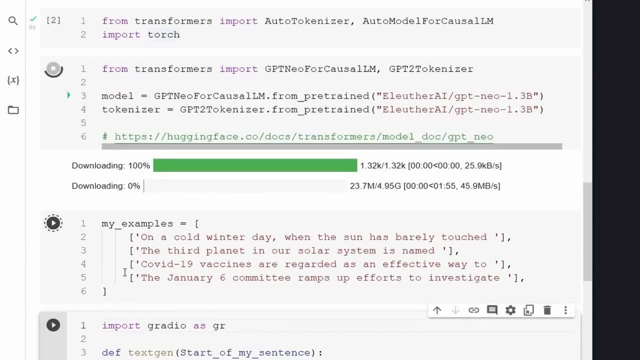 examples you notice from the last video. These are the default beginning of the sentences that we want to have our AI NLP text generator acting upon. So as you can see now I'm downloading here GPD Neo 1.3 billion free parameter model. 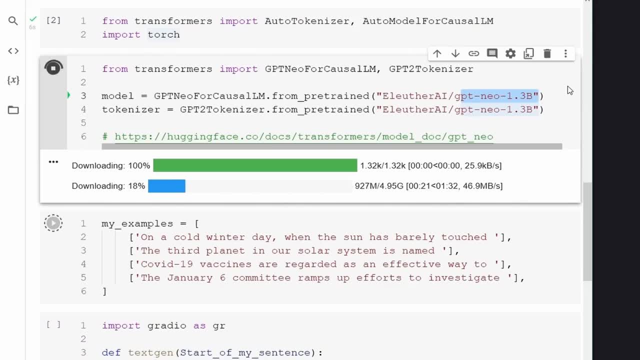 So the smallest model I am aware of is GPD Neo. And you might ask, hey why you don't go for 2.7B or the 6B model. Well, have a look about the RAM that I will need to run this. Remember this is my free CoLab notebook. 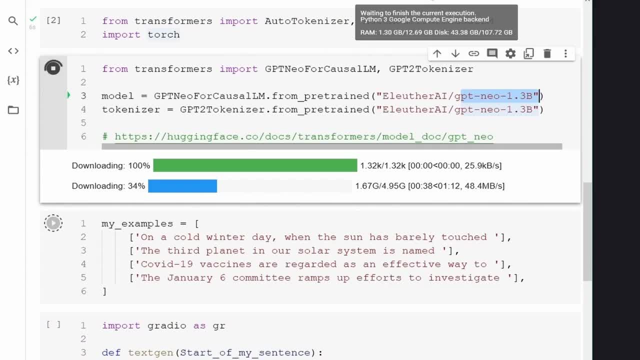 This is not the CoLab Plus or anything. I just have 12.7 GB of RAM available to me. And as you see we are downloading here now close to 5GB of RAM. 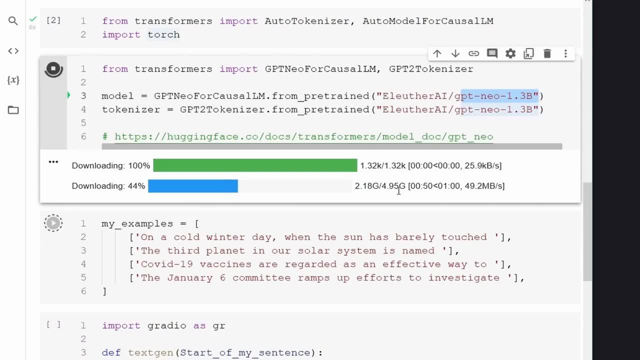 download file. the GPT-Neo 1.3b model. This will take another minute or so. And then what we do again, we import 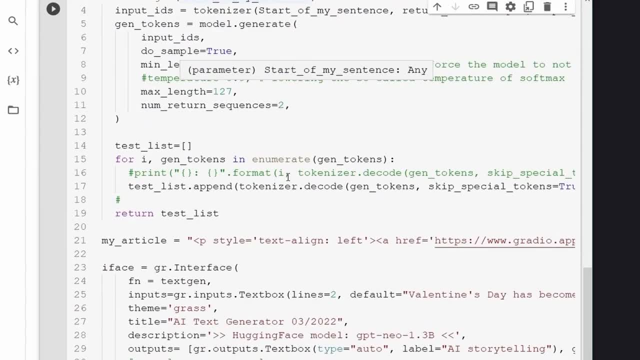 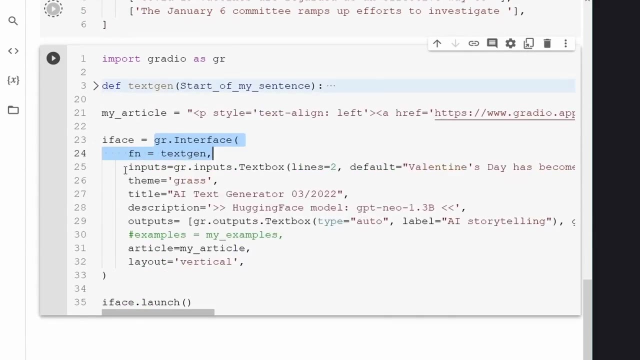 Gradio. And as I told you, we have always the same if we use Gradio. Now with the interface functionality, we have at first a function. This is our defined function. I define the function here. We'll come back to this in a second. Then we have our input and we have our output. 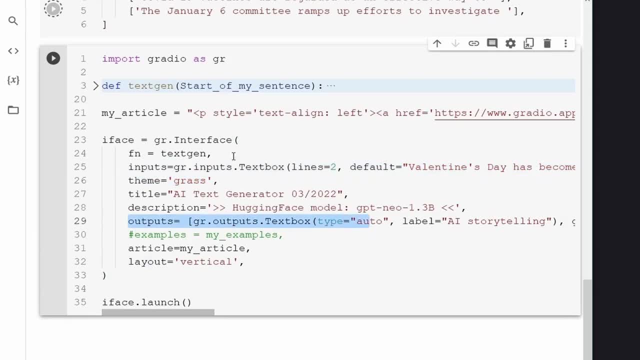 And those three elements are always the same. So the function we're going to talk about, the input is a simple text box. And there is maybe even some default values. This is a good 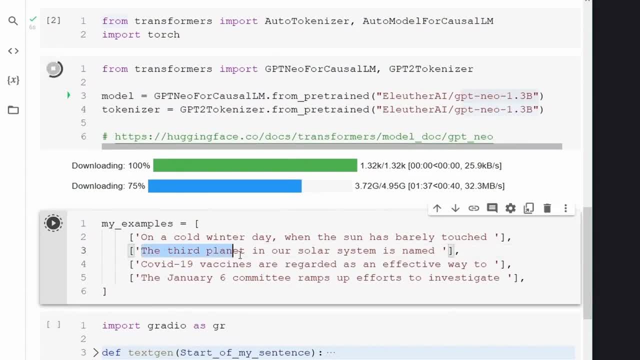 idea. Maybe you want to change this. And we say that's our plan. Our system is named. Just copy this. 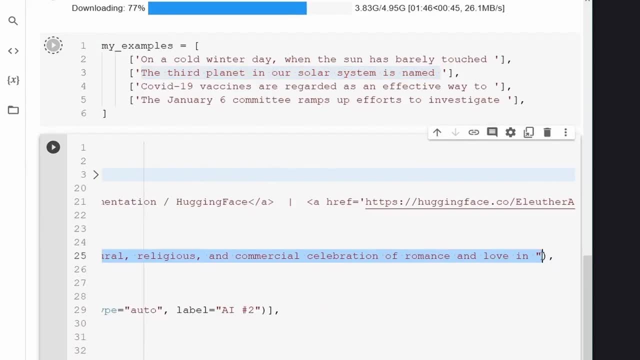 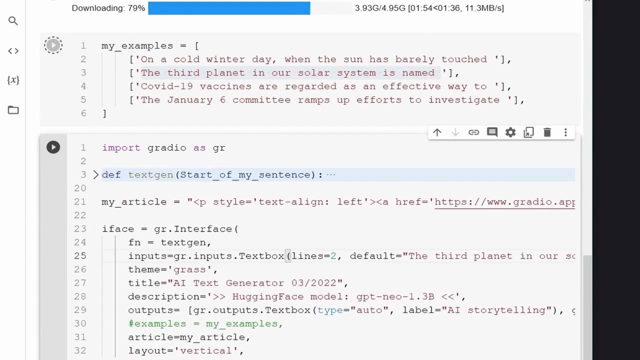 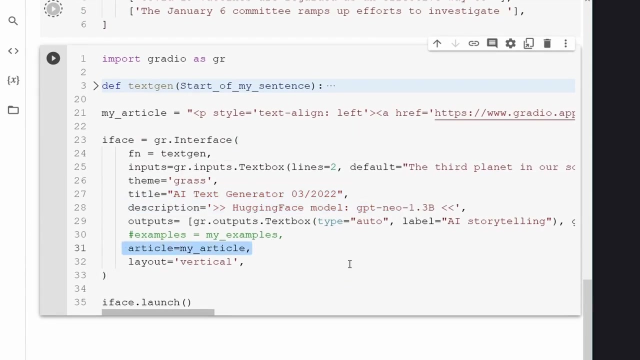 And we make this a default value in our text box. Come on. While we are waiting. Then we have the title. We have a description. We have an article where I have to link to this 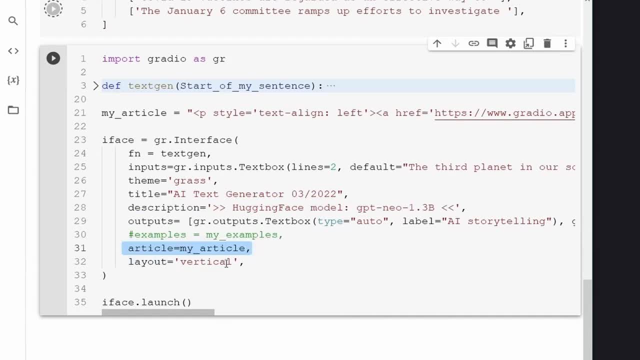 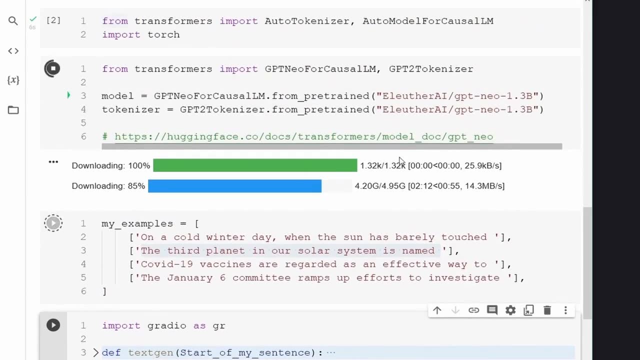 model that I use. And you have an option for the layout vertical, or you can have a horizontal layout. So we are here close. 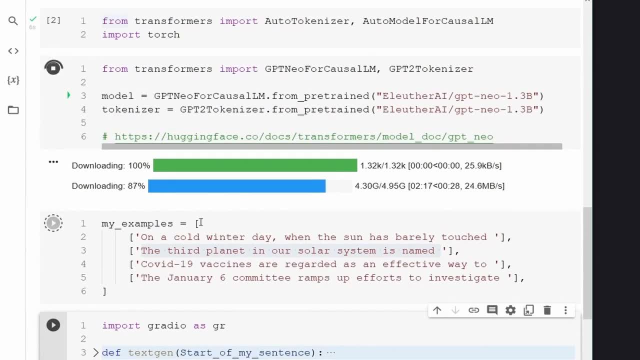 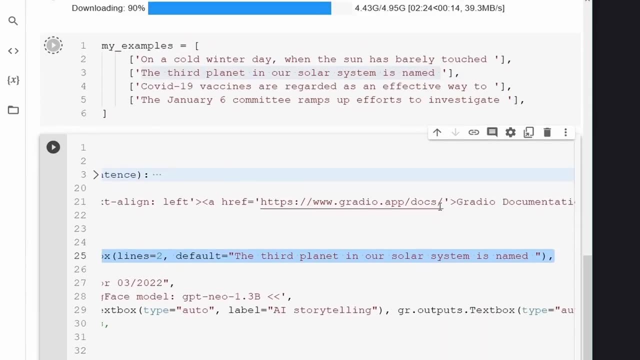 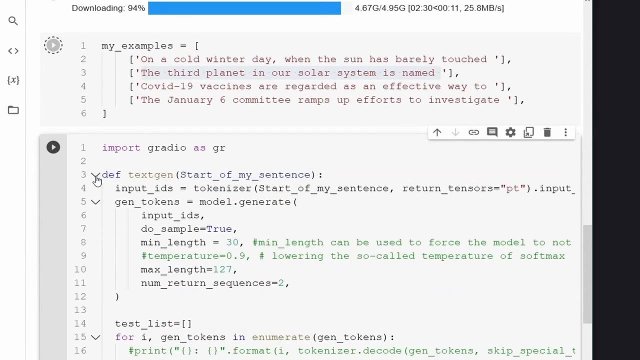 Let's go to finishing the download. 86%. Come on. And as you can see here with the input, I went here for a default one. Let's try this one here. Come on. And while we wait, the function I defined. 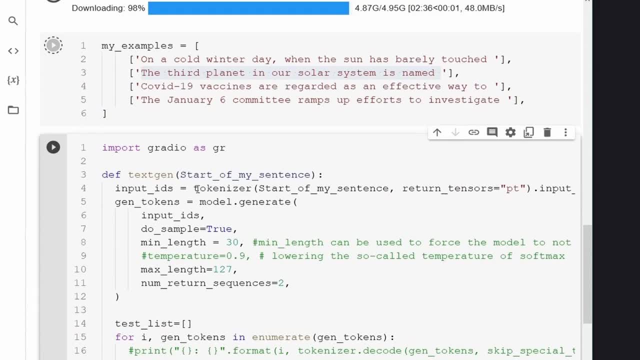 It is very easy. I say, okay, my input ideas. I have my tokenizer. I'm working here on PyTorch, of course. And then, as you know, from... 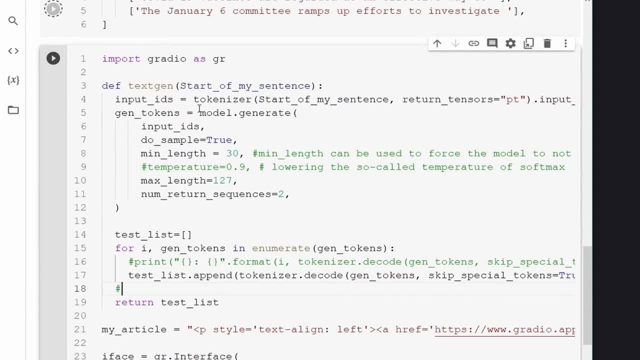 your typical transformer Python code, you have your model, your generate command. You have your input ideas. You have now, this is why I do it, a minimum length and a maximum length. I want to have a minimum output length and a maximum output length that I can take care of. I don't just want half a sentence as a response, but I want two or three sentences as an output of the model. 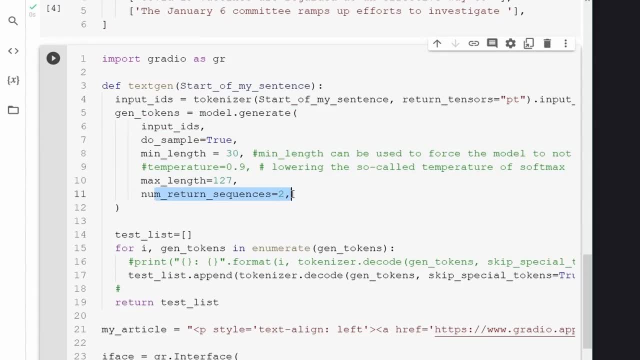 And then I can go and I say, hey, I want to give it two tries. So give me two examples of a calculated answer from your model. 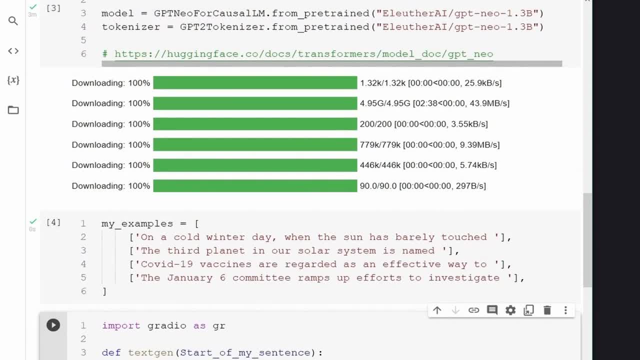 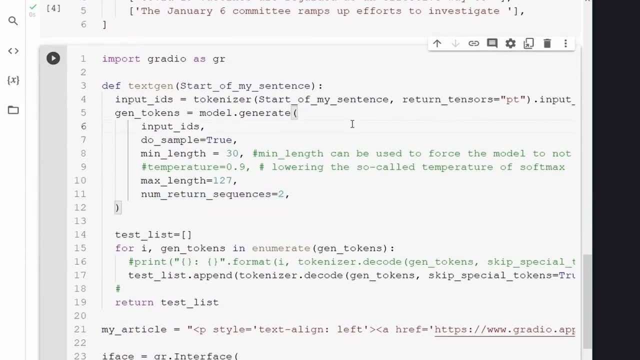 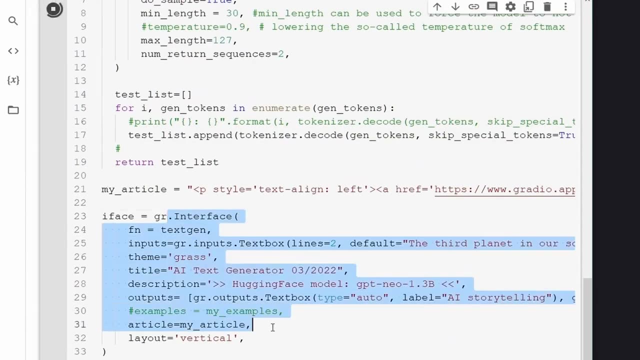 And this is it more or less. And as you can see, we have now about 6.4 gigabytes or half of our RAM is now in operation. And then we just start here. We launch our Gradio interface. This is it. And have a look at... 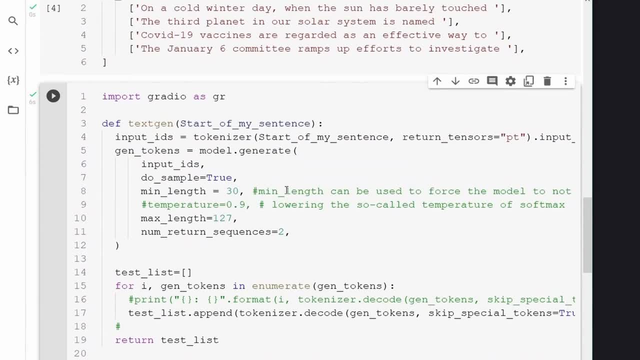 This is it. Beautiful. This was so beautiful. Last time it crashed. Okay. Presentation. Beautiful, 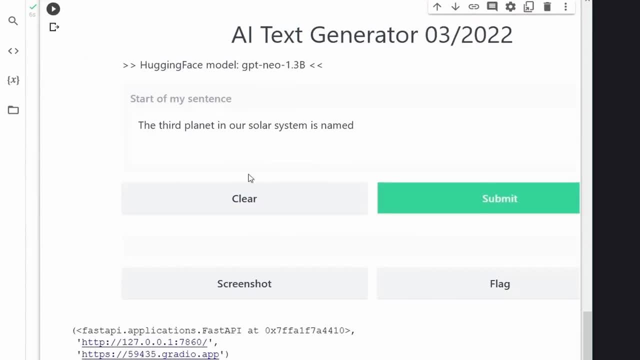 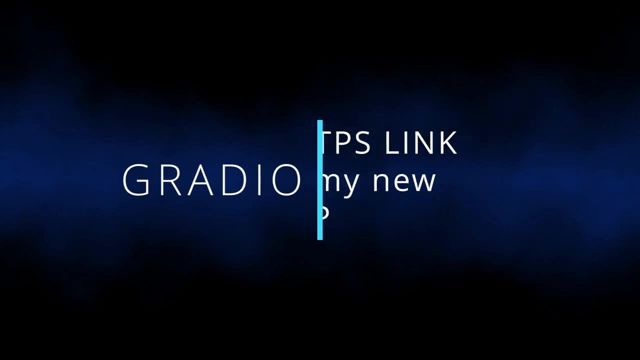 beautiful, beautiful. We have now in Colab inline our AI text generator. But hey, we say, let's have a look at this in a more closer window right next to our code. So here, as you can compare this, 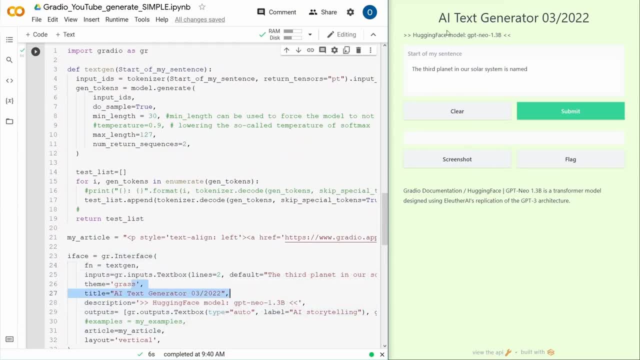 we have our title. We have our... 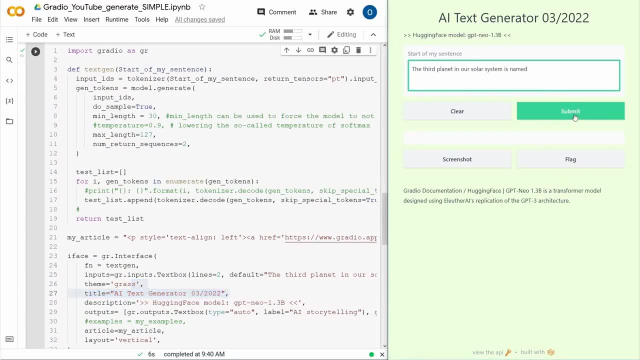 This is it. This is our title. This is our comment. This is our comment. This is our comment. The third planet in our solar system is named submit. And now we are running now this on the Google Colab notebook. 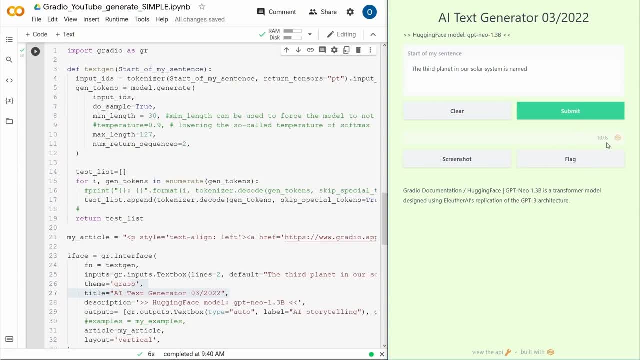 And as you can see, it takes, of course, longer because I have just a plain old Colab. No particular pro version or anything of this. 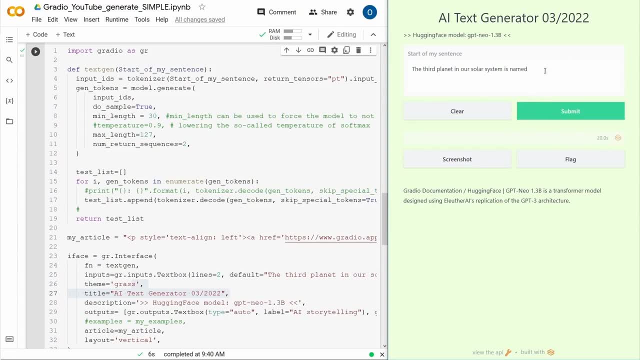 So depending on the complexity of your sentence, we will have to wait quite some times, 25 seconds or so. 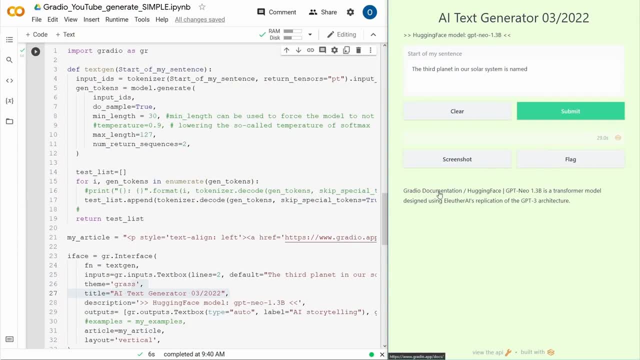 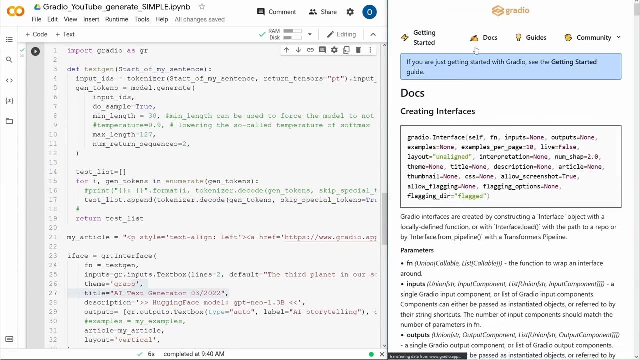 already and as you can see i told you we have here the graduate documentation you can have a link here in your app if you click at this you get here the direct link to radio and the other thing i 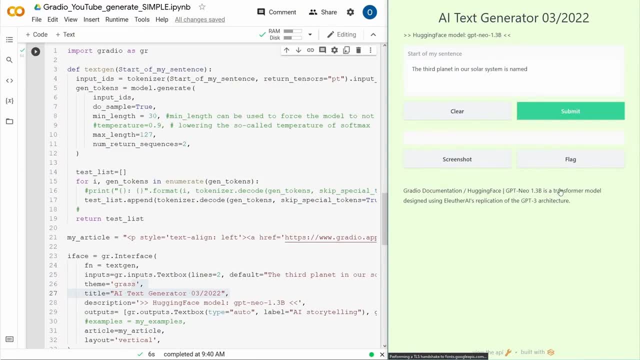 have a link integrated is the gpt neo model this is of course the transformer home page from the 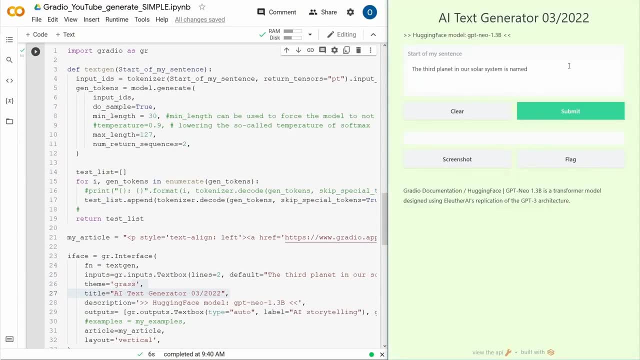 from hugging phase but let's go back let's have a look and yes great i finished this my goodness 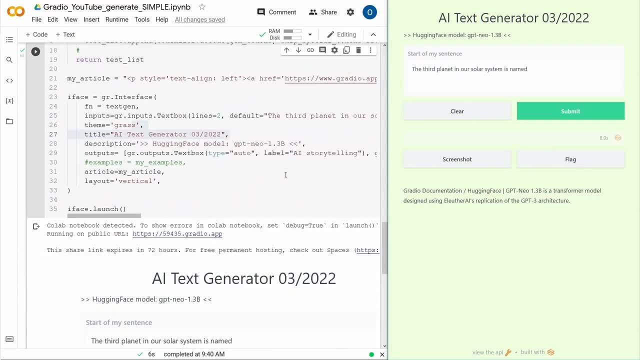 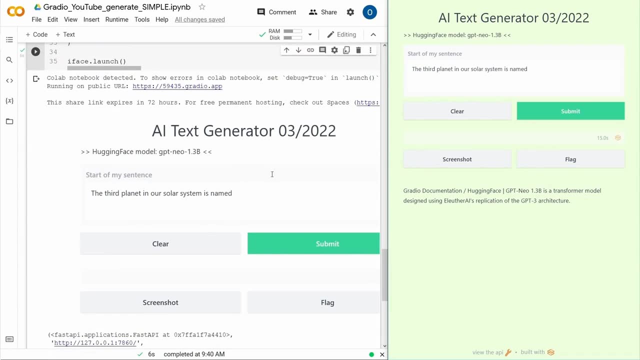 sync this would be highly appreciated well yes yes yes and as you can see here either you use 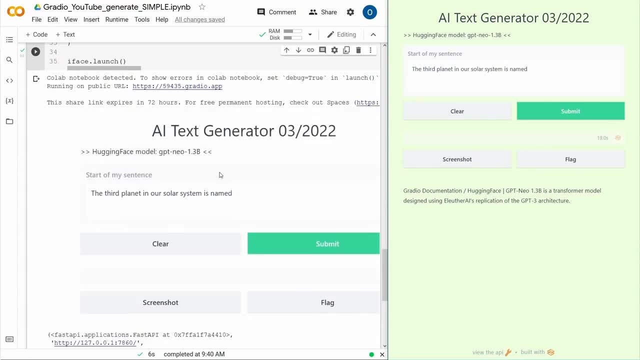 here the application here directly in collab or if you want to send it out for somebody no 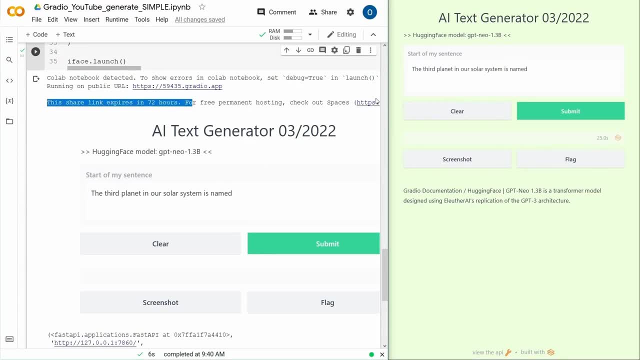 problem at all they say that for free permanent hosting you can of course check out spaces from hugging 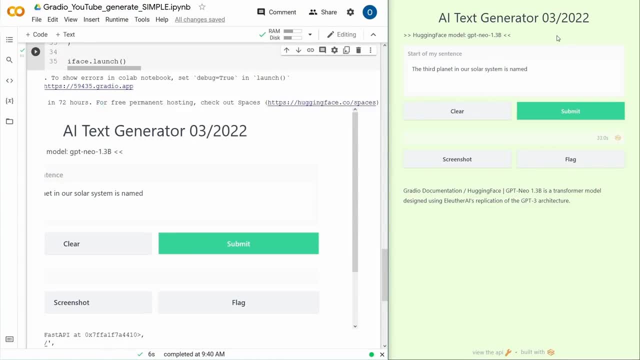 face where you can post your radio generated hugging face space model if you want for free 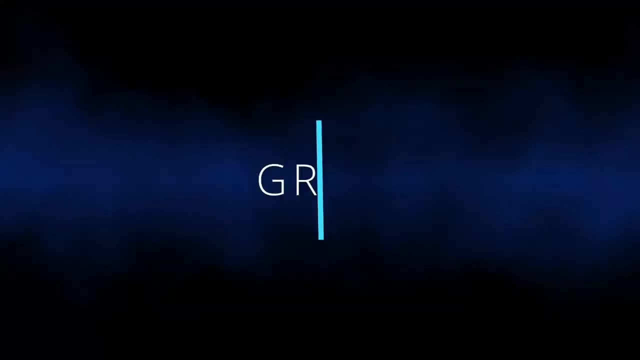 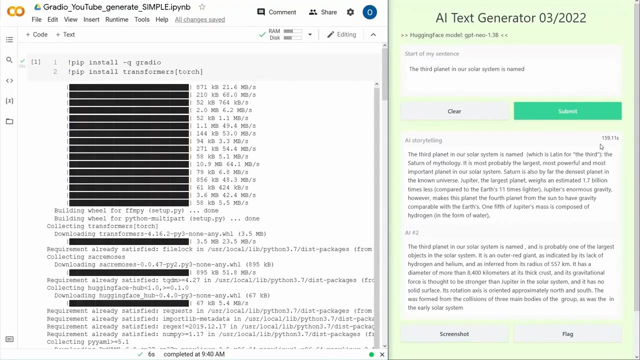 currently march 2022 and finally after 159 seconds we get a result so let's 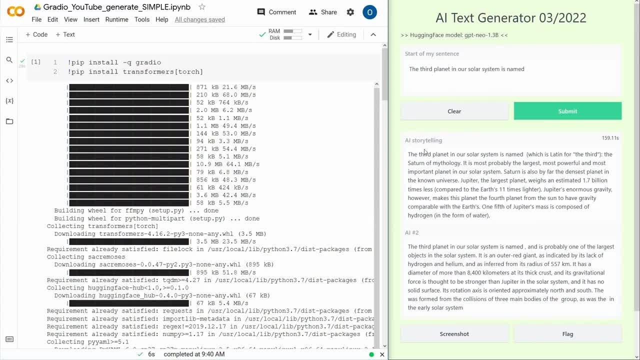 have a look at ai storytelling by our nlp model from hugging face the third planet in our solar system is named which is latin for dessert the stature of mythology 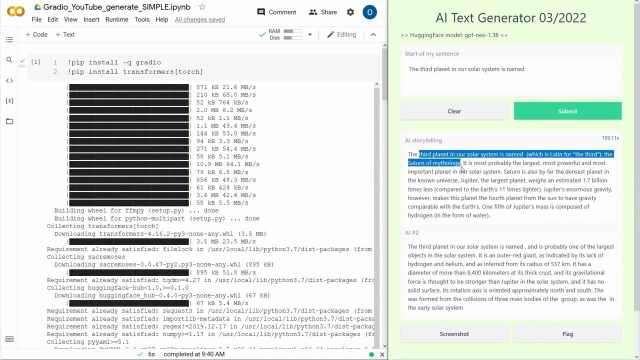 well factually i would say this is not the right answer but it is a nice answer it is not true but we put some information about whatever they think 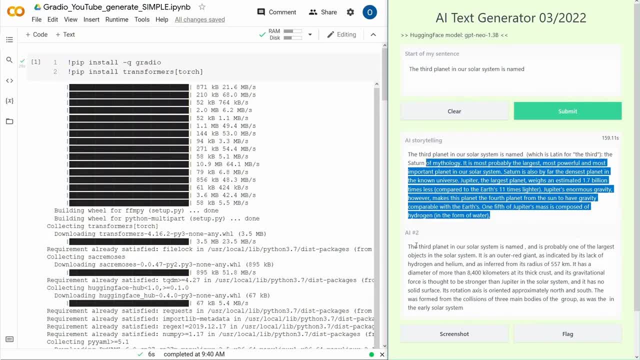 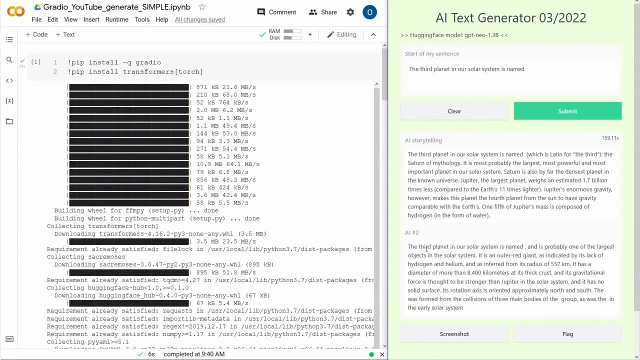 might be a nice planet now let's have a look at the second answer provided by the same model by just tweaking some parameters is named and is probably one of the largest 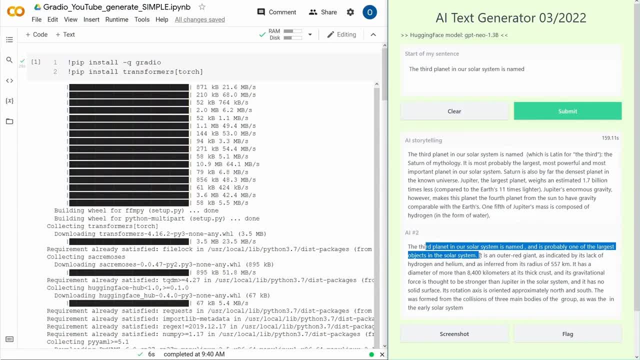 object in the solar system no definitely not jupiter and saturn are much bigger than earth 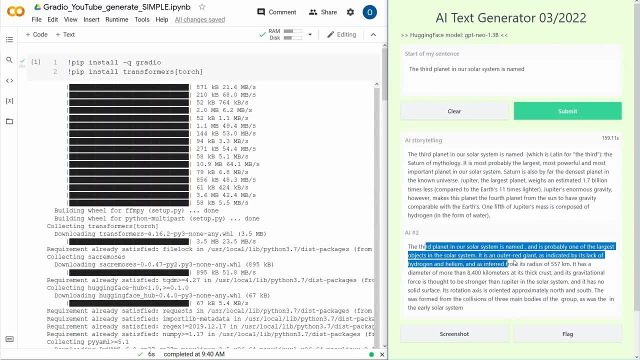 it is an outer red giant and has in for 557 kilometers is the radius of the object no it has a wow so the radius is 557 k and has a diameter of more than 8 400 kilometer 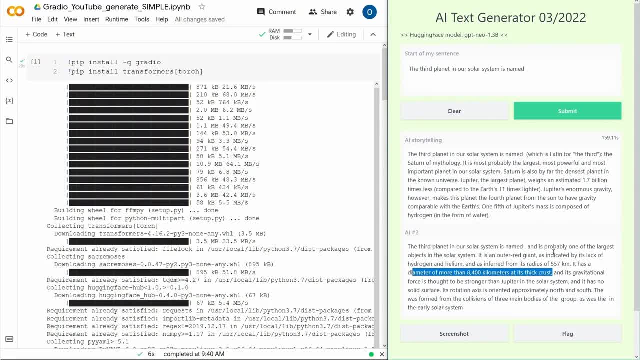 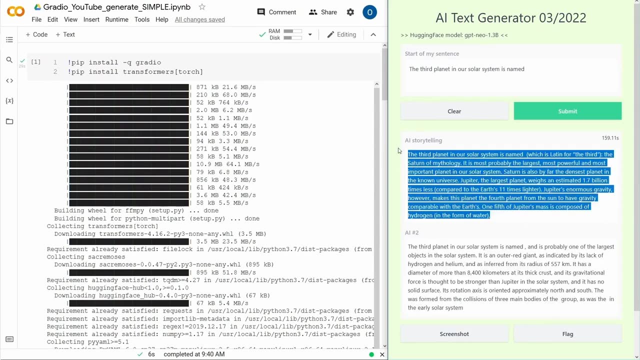 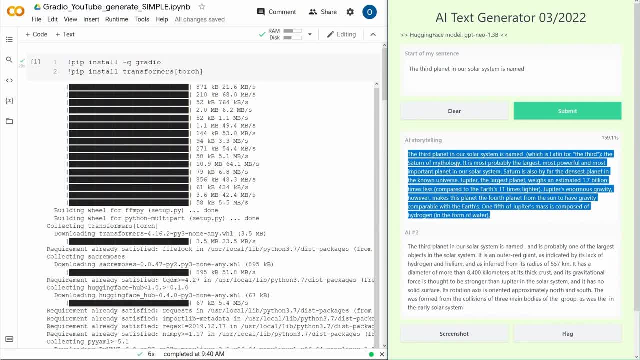 depends so much on the quality of your input data and of course on your system 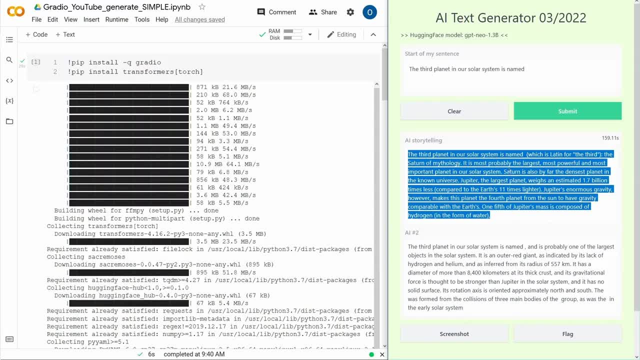 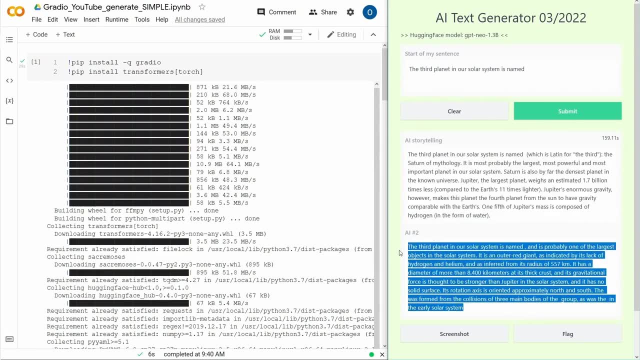 so maybe the next time or in the next video i will show you how to fine tune the system how to optimize the system what can we do with this system that it 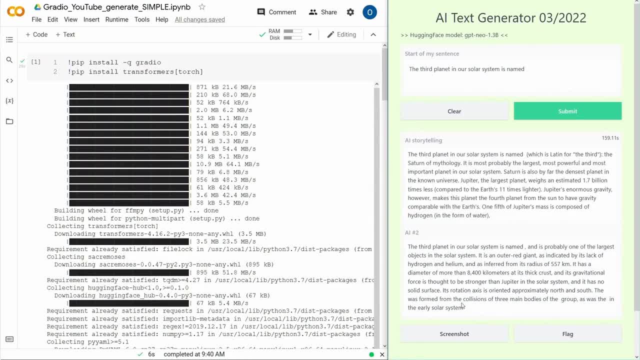 performs a much better way i say thank you for this part of the video and i see you in the next one you 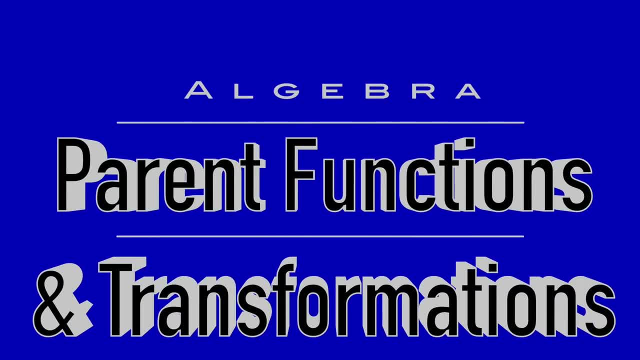 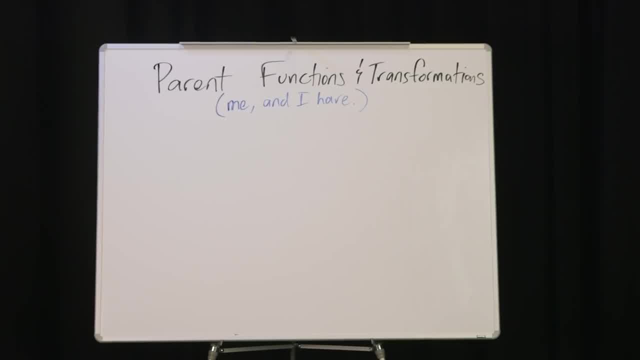 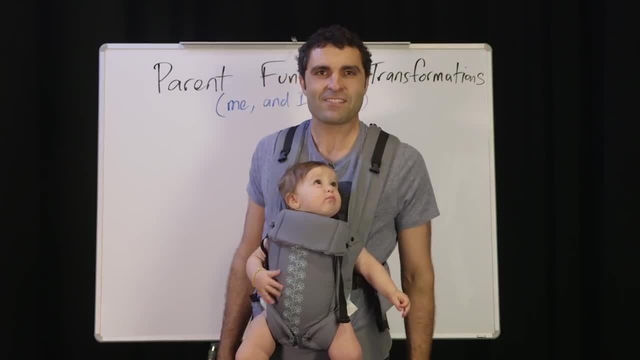 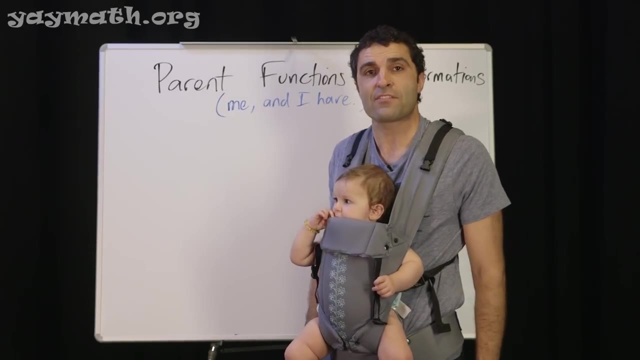 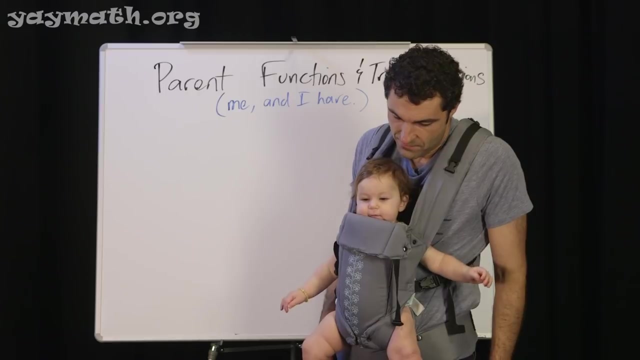 Hey everyone, I'm Robert. this is Yay Math, and this is my little baby girl, 8 months old, and this is just another standard day of mathematics within our household, So we thought we'd share it with you. Want me to teach you about parent functions this time.